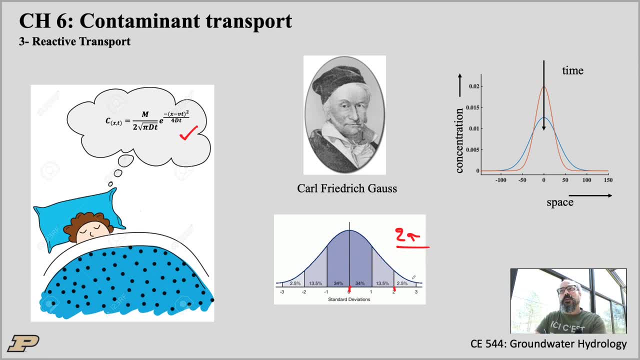 fundamental characteristic of a bell curve that we use to calculate dispersion coefficients. And finally, here on the right-hand side, right here, you can see how this bell curve, this fundamental solution, is plotted in space and time, right. So, space on the x-axis, concentration on the y-axis. 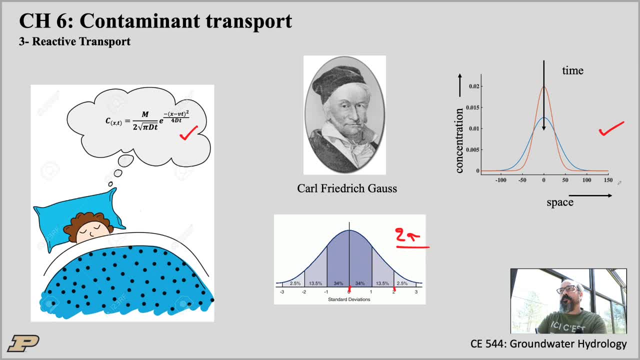 and then finally, time, you know, on the third dimension. So if you have a pulse injection, a delta function as the initial condition, then over time the dispersion will just spread that pulse away. Okay, and again, the dispersion is basically what makes this spread out over time. 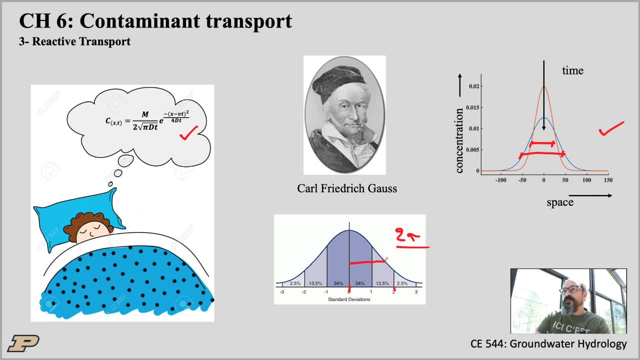 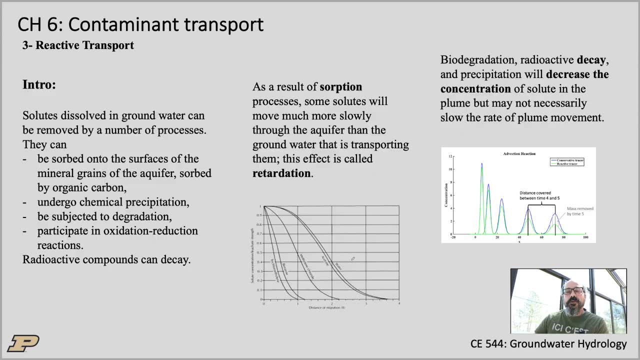 Again related to, of course, the bell curve here and here. Okay, so there was the quick review from last time and today. finally, we want to know what happens when we have different compounds in the mix. So this intro- again, this is taken from Federer, essentially, And a lot of the illustrations from today are. 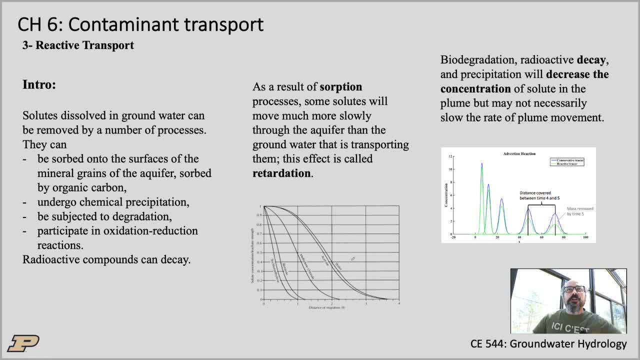 from Federer, per usual. And of course, solids dissolved in groundwater can be removed by a number of processes, right. So the first one, the one we see today, is sorption. right, So they can sorb to surfaces of the soil matrix or the formation matrix, right, Grains in the 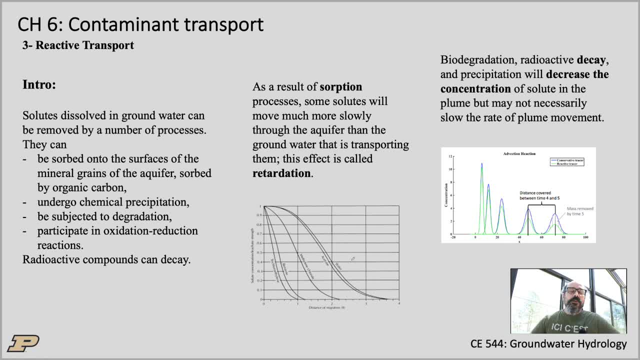 aquifer For organic compounds. we'll talk about them a little bit at the end. but they can sorb, you know, on organic carbon. So if you're in a soil you know a lot of organics are going to stick to organics and then they'll have retardation as well or they'll be slowed. 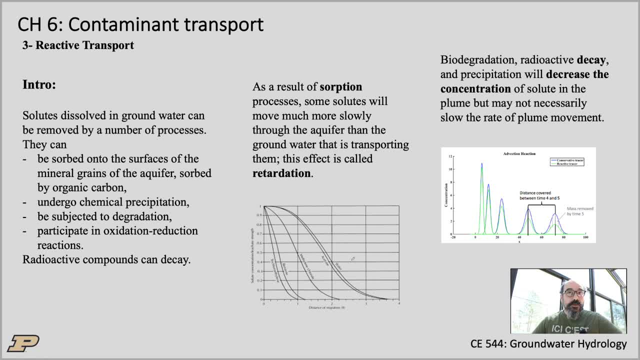 down. There can be chemical precipitation, right. So if you have a salt, for example, that starts precipitating, then it's removed from the plume. Degradation and oxidative reduction are aspects we'll see on the next lecture, And then, finally, radioactive compounds. 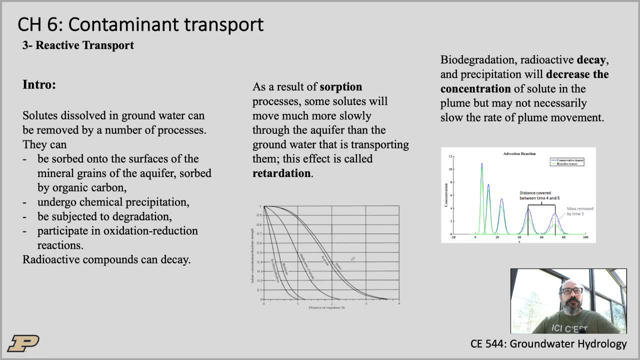 right And just decay at their own pace, so they just disappear. So again, all those chemical reactions essentially remove mass from the contamination. And again today we want to pay particular attention to sorption, right, So sorption basically is a process where molecules 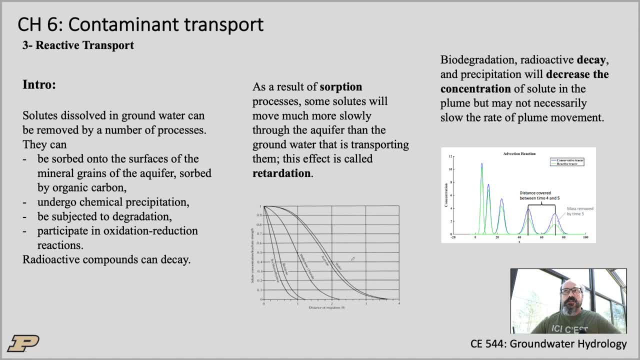 will stick to the surfaces of the soil matrix. Thereby they're removed from the moving plume and eventually they can be re-released. So if you have a molecule, that is, that sticks to a particle of soil over a mineral and 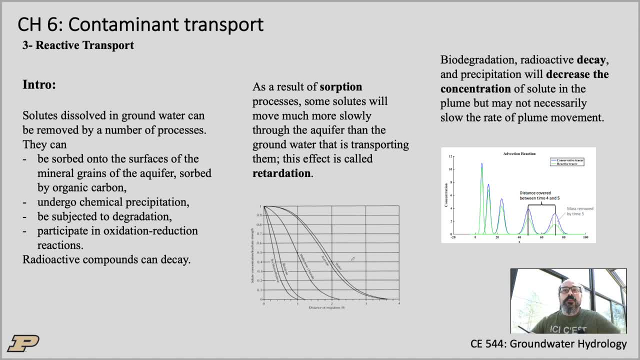 then is released later, right. Then it starts moving later. So the overall effect is to slow down the contamination Again, biodegradation and radioactive decay can decrease the concentration, and that's the object of next week's lecture. So again, here down here is retardation. You can see the water at the top and then 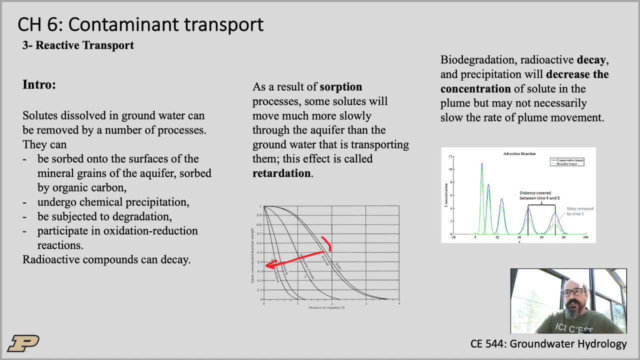 more and more. you know retarded species or delayed species. So if you have again an initial pulse, you know the water is moving this fast, but then different compounds move slower relative to each other And here on the right this is the decay. So you can see. 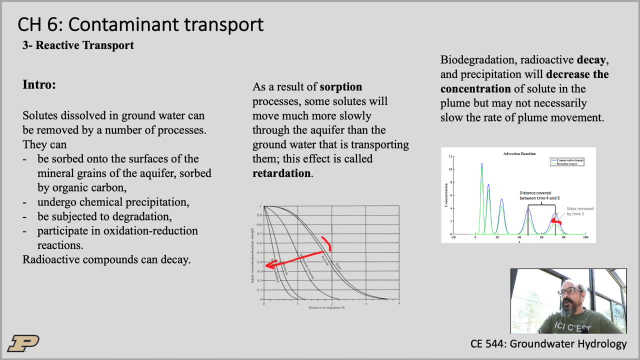 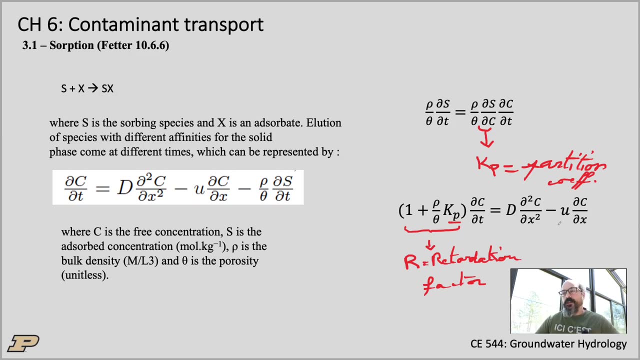 here we have missing mass, right. So it's been degraded, So it moves at the same velocity as the water, but now mass is removed and you know we don't find it Okay, so diving into the sorption aspect of transport. So again, this is this first equation on 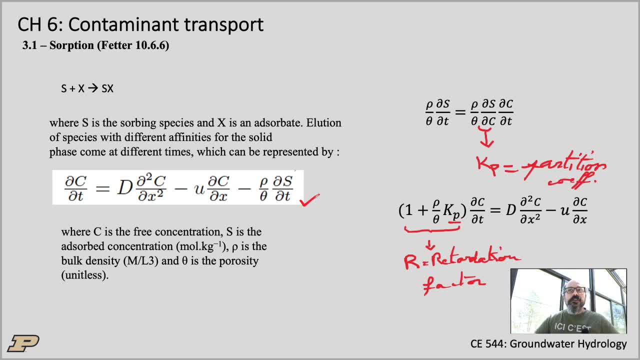 the left here. This is your transport equation from last time, so advection-dispersion. But now we have an additional process which is basically the retardation right. And importantly is that last term dS dt right. So S would be the concentration of the sorbed species, right. So again, S would be a concentration. 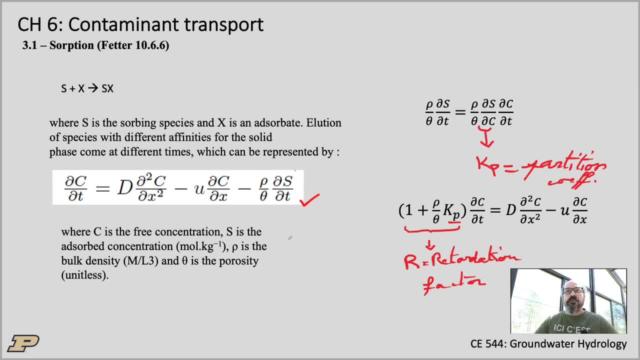 in mass per mass. okay, So this is different from what we've seen before because, again, you know, if you want the concentration of something that is stuck onto a grain, onto a mineral, now the concentration has to be, you know, mass per mass of mineral. right, there's no volume of water. 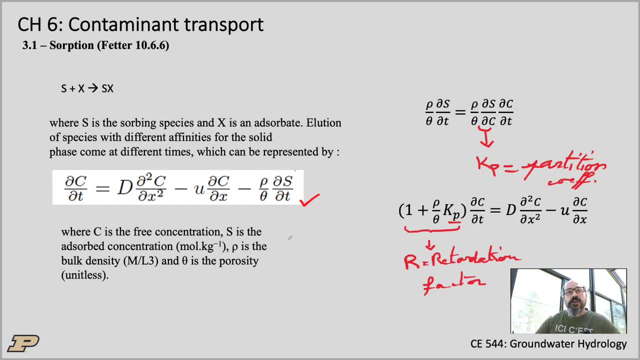 or volume of fluid, because obviously it's a solid. so now we're dealing with concentrations in mass per mass and that's why you have that, that factor here. that includes density, right. so this is mass per volume and this theta is the porosity. all right, so theta here really should be porosity. I mean, it's the same. 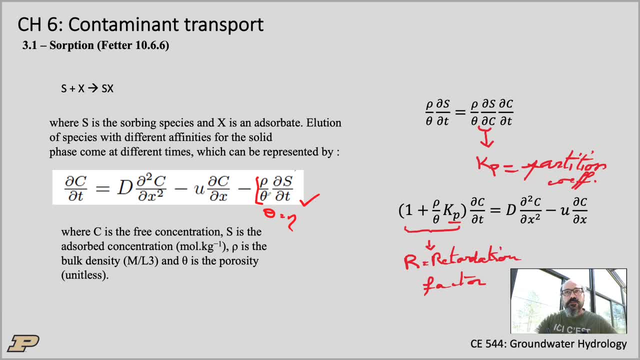 thing, but theta is really the saturated content. so if we did like beta zone hydrology- right, theta is a more general term than porosity. but if it's a saturated aquifer, like the ones we've been we've studied in this class, then you know theta is basically the same as porosity. okay, so again you have density. 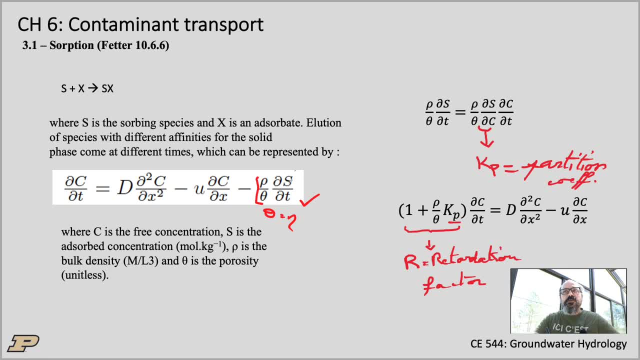 and this is because now our concentration is in mass per mass. so if we wanted you know mass per volume, then we would need to know what is the bulk density of this aquifer. so now, when we look at this, you know the units are consistent, but we 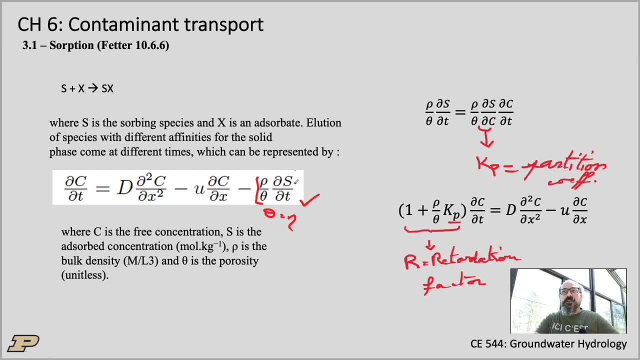 have the concentration of the absorbed, of the absorbed substance in mass per mass. now one way to transform this equation, with you know, into a retardation factor is to look at the chain rule, right so here on the right hand side. so I extracted this term right here. 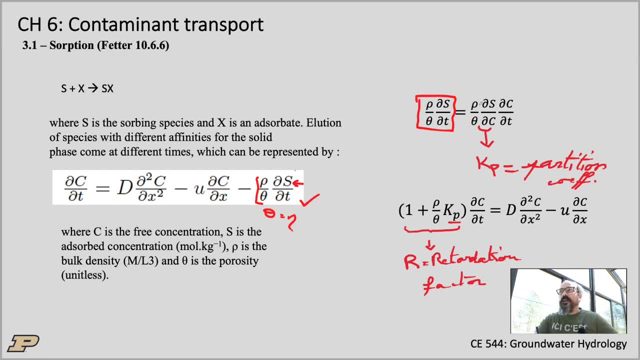 and just rewrote it the same, but now extracting that dcdt so that we have the same expression that we have on the left hand side rate. and now we can see that in the equation, now we have dS dC appearing right. so again the change of 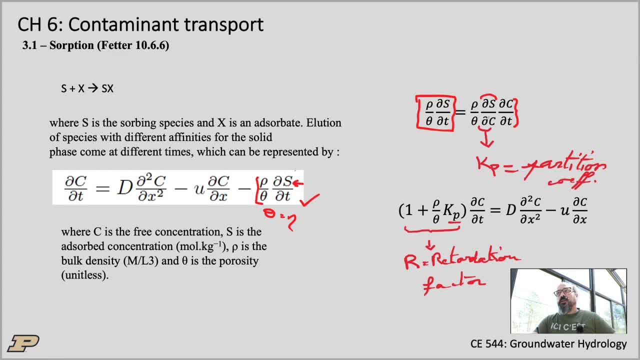 absorbed species per change in bulk concentration, right. so this is really intuitive, because that's what we call a partition coefficient. but if you think what that is right it's, if you have a plume of a contaminant passing through a formation, you know, the higher the concentration, the more sorb species you have, right. and then later on, 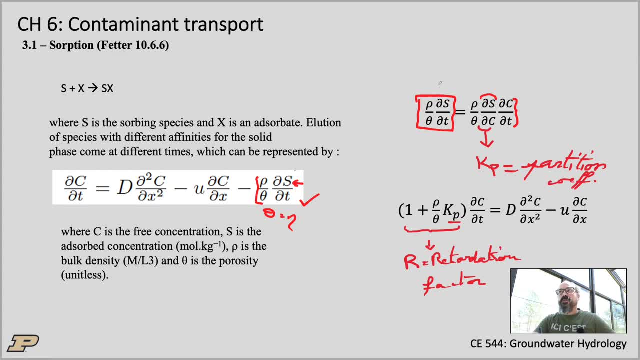 when we have clean water basically coming through and the, you know, most of the plume, most of the mass is gone and now we have at the tail, we have, let's say, clean water. that clean water is essentially rinsing or cleaning up right the rest of the rocks that still have a bit of sorb stuff. 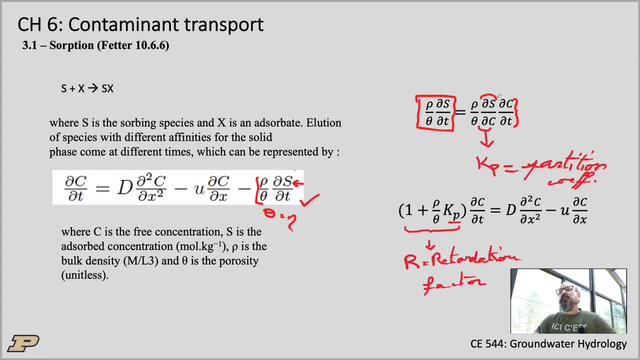 right. so it makes sense that the amount of sorb concentration, the amount of sorb material, should be proportional to the concentration in the plume right. and again, this is what we call a partition coefficient, literally, you know, if you look at the etymology or the meaning in english. right, we're. 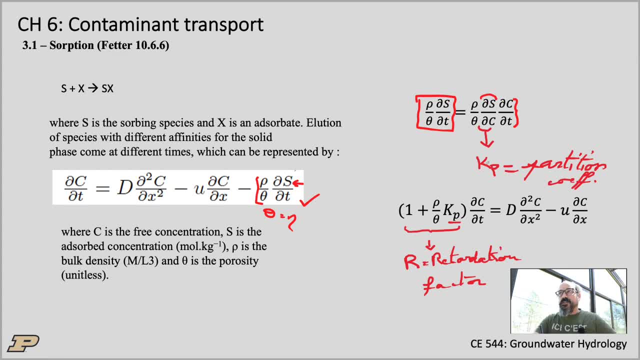 just partitioning that plume into, you know, some dissolved stuff- that's c- and some sorb stuff, that's s. okay, so now we can reshuffle all of that right. so now we have dc dt. so if we replace, you know, this whole ds dt by the expression on the right hand side, now you can see that we can shift everything to. 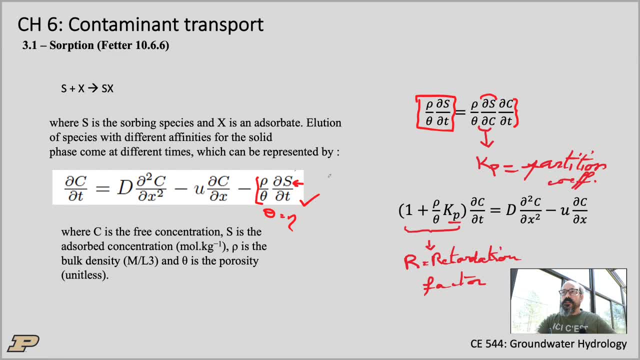 the left, right. so now we have something dc dt here, right, blah, let's call this whole thing blah. so this is blah here, right. so blah, dcdt. now we can shift this on the right hand side and we can see that we have dc dt. we can factorize dc dt out and now dc dt is going to be, you know, factor one plus blah right. 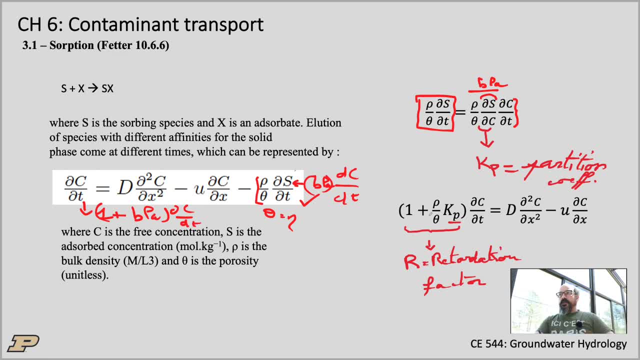 and this is what's here. one plus uh, rho over theta, again theta or eta, you know, like porosity rho over porosity times, kp partition coefficient. so this is what we have here now, this whole bit here. that is the factor of dc dt, we can just call that r. 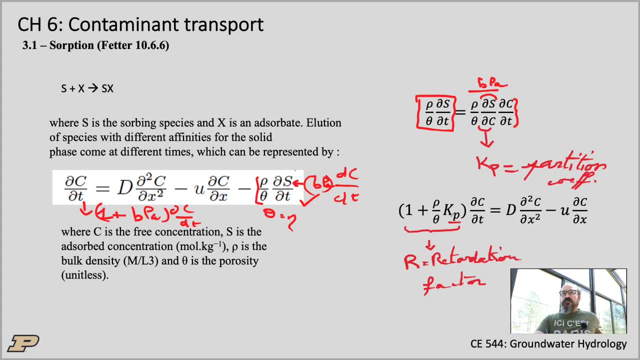 and call this a retardation factor. so now you can see that you know, after this bit of math, you know we have a very easy, simple solution or simple equation. i should say that is pretty much exactly the same as before, except now we have a retardation factor in front of it. so you have it here at the 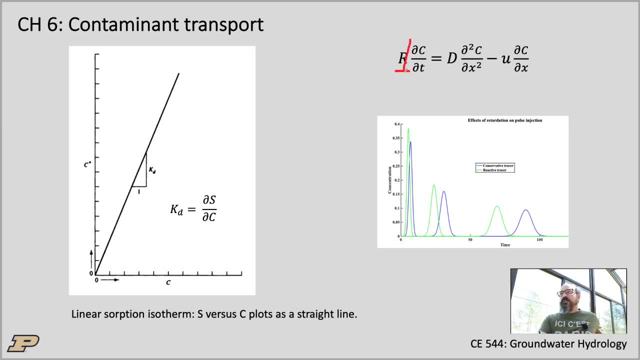 top right, the retardation factor. so now, after you know this bit of math, you can see that basically we have exactly the advection dispersion equation from before, and then there's a retardation factor. you know whatever that is we just saw. but there's a number here that just modifies dc, dt. 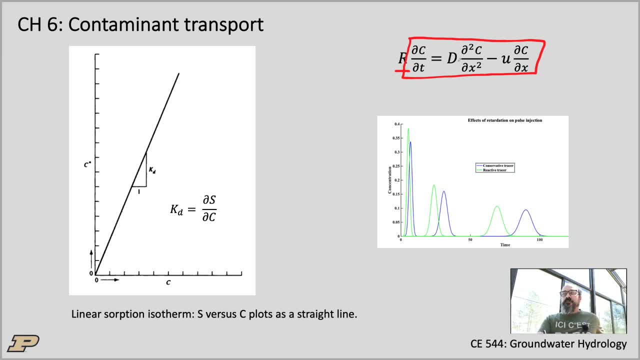 an important aspect to understand here is r is you know the factor? so it's obviously dimensionless. if you shift it back to the right hand side right now, you can see that the reactive dispersion coefficient is d over r and the reactive advection or velocity is u over r, right? so if i shift this to the other side, then we have dc. dt equals d over r. 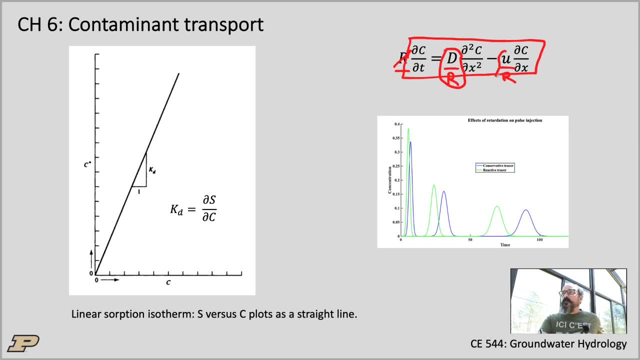 minus u over r. so all retardation does really is modify our velocity and dispersion, right? you divide this by r and you get the actual- you know reactive or retarded- velocity and dispersion. so very simple, and you can see the effect here for a pulse injection after some time. so this is 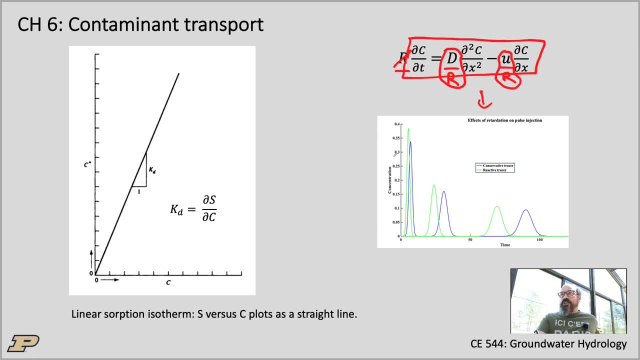 one week, one month and three months, you know, after an injection and you have the code. you'll have the code in your folders and i'll show you in a minute, but you can see that basically, what happens is the retarded species is just, you know, slower to reach some uh location. right, this is again. this is. 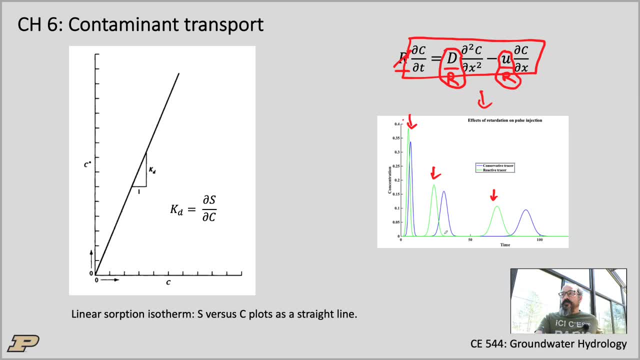 time here. so this is, um, yeah, seven days, uh, 30 days and 90 days, and here the velocity is like one minute per day. so you can see that you know the mean, uh, the mean time of the conservative tracer is. the mean time of the conservative tracer is just, you know, the number of days, basically. 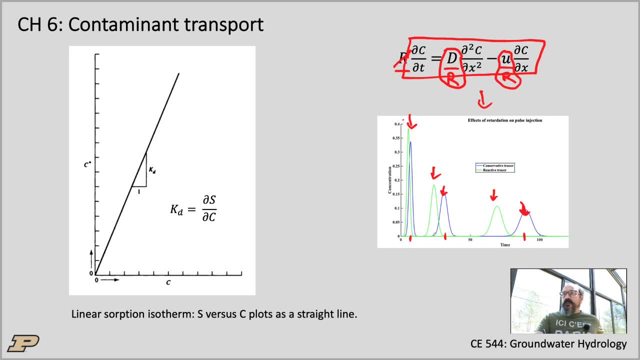 because it's one meter a day and here, but then the at the same time right. the reactive tracer is not as far right, so it's going slower, basically at 90 days. it's only, you know, partly through the transport. here on the left hand side you have what we call the isotherms. 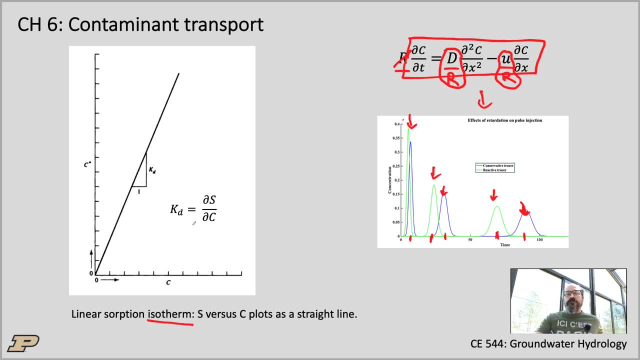 and this is an important term- for sorption. we'll talk about those in the next few slides a lot. but for a linear sorption and i- i make a distinction in a minute. but again for a linear sorption, by definition, we've seen that k- well, kd or k p partition coefficient or this is: 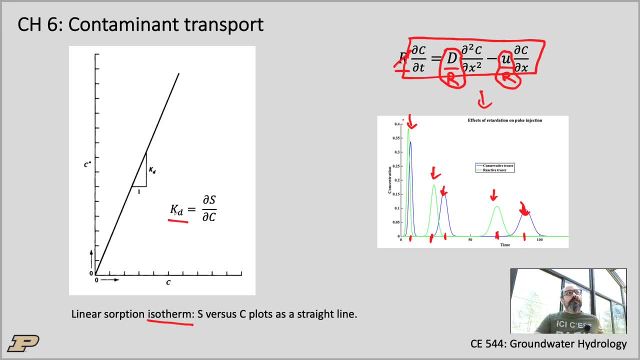 the way that we call this for. uh, i can't remember what the d stand for. anyways, it's the same as the previous one, right? so we we define it as the concentration, the change in sorbed species per the change in bulk concentration in the fluid right, and if it is linear, right, because the definition is this that we gave. 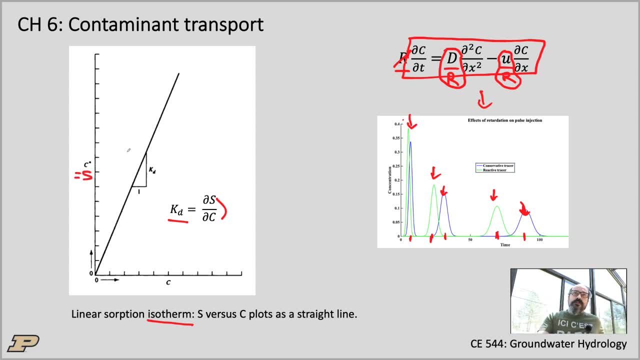 before. this is basically just the slope of, and again, c star here equals s. this is just a different. make the difference, you know, to really emphasize that this is the sorbed species, but in the feathered he uses C star for the same thing, right? so anyway, 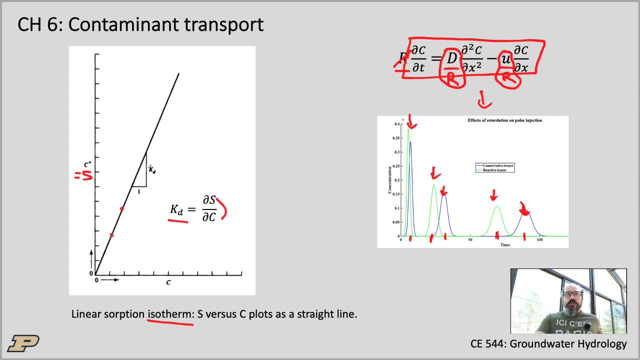 so if we take a plot of the sorbed concentration versus the bulk concentration, so the concentration in the fluid, now you can see that this plots on a straight line because it's linear right and the slope is KD by definition right, just like we've seen before. so if we have this data, then we 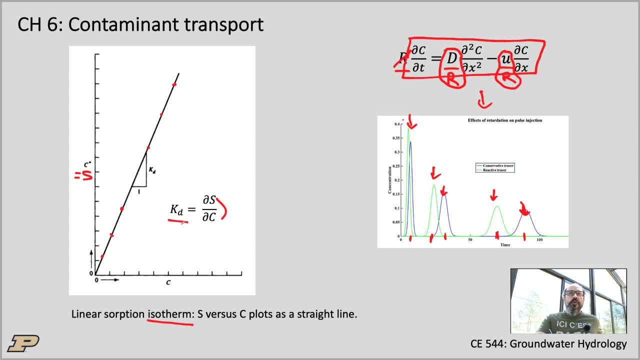 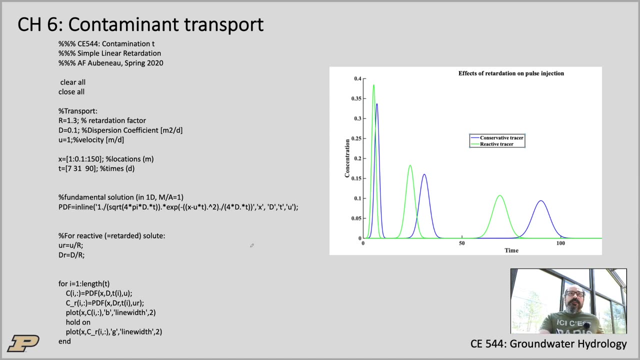 can just take the slope and know what KD is, and obviously rho and theta, or the porosity and the bulk density, should be known. so now we have everything to actually calculate the retardation factor. okay, and again, this is the same plot as before, right where we can see. so here I'm putting the code so I can. 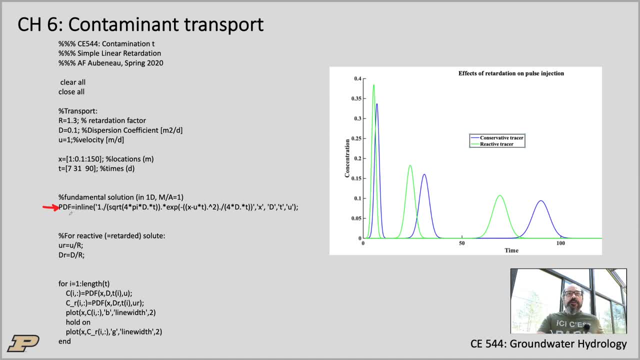 emphasize how easy this code is right. this is what I call PDF is just the solution to the advection dispersion equation. right, ADE? right? so you can see that C at t equals, if you remember, M over square root of 4 pi dt exponential minus blah, right? so this is our fundamental solution that we wanted. 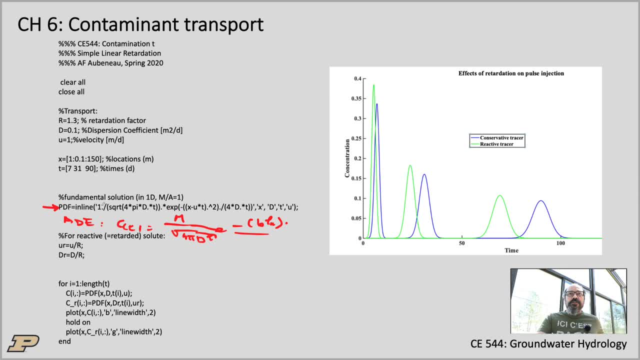 to remember, and you can see this is just the MATLAB version, right? so now M is 1, just if we make it a PDF, right? so it's just 1 over square root of 4 pi dt exponential minus blah, right, and so this is just the function. so all I did here. 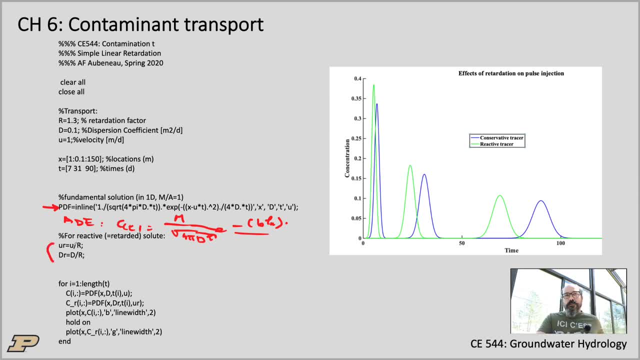 is for a reactive solute or for sorption. right, all I do is divide the velocity by the retardation factor, divide the dispersion coefficient by the retardation factor and then run the exact same equation- right, but with those modified velocity and dispersion for the reactive. so the blue lines are just. 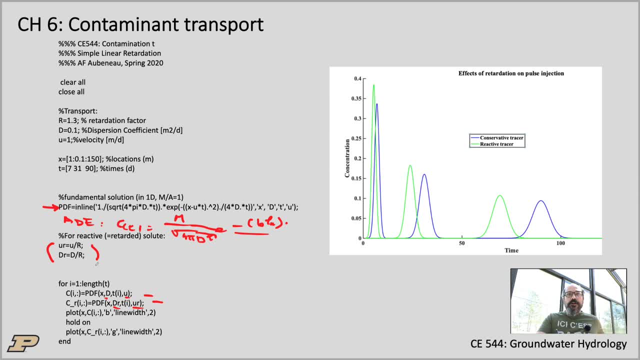 you know the original velocity and dispersion and those green lines are the modified. you know, divided by R, velocity and dispersion, and that's really all it is. if you have linear retardation, you know you just have that retardation factor, you just plug it in and that's it. that gives you directly. you know the. 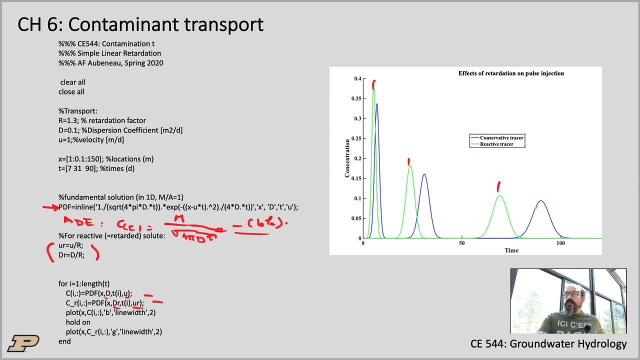 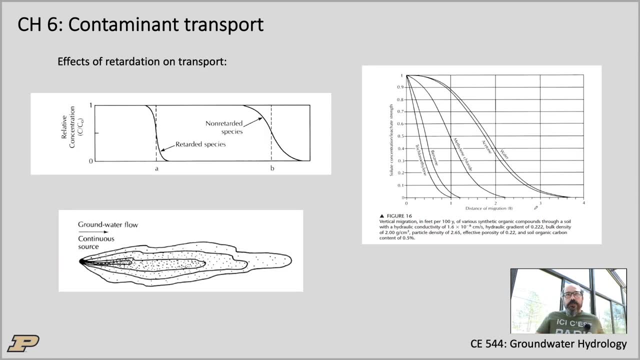 slowing down of the plume compared to the water, compared to the conservative transport which is in blue here. okay, now other illustration right of what retardation does in other boundary conditions, if you will. so right, here is the right now. I've just illustrated with that simple pulse initial condition. we've 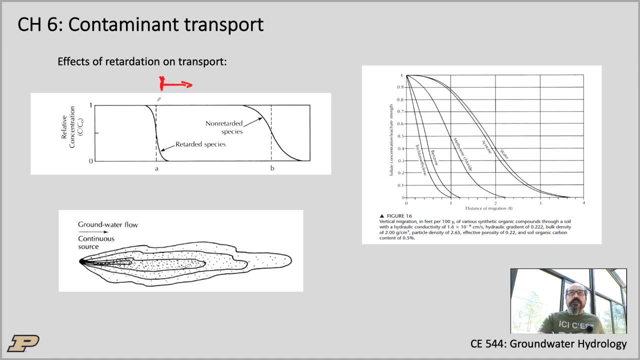 seen last time, when you have a sustained source right or a front moving right, you can see that the difference in arrival time again is just the same as the pulse, but just with a different front here illustrated. so this is for a square input, basically, or continuous input, and you can see again that the non retarded 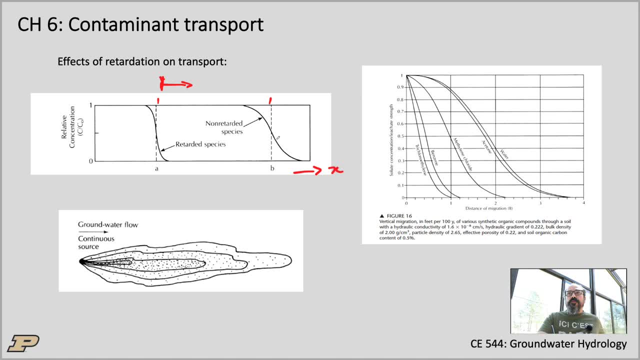 species is much further out, right, so this would be distance now, right, so the front is much further out, so this is the distance now. so this is the distance now further out that for the conservative, for the water, basically for the conservative species, than it is for retarded species. retarded species, if you will, you can see here. 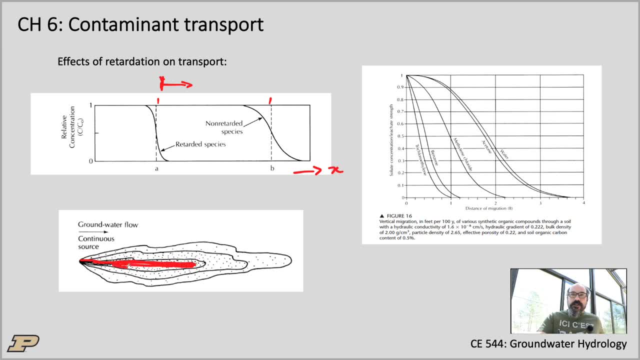 down, down, down in that illustration. for example, this: you know, this middle plume here would be for the retarded species, right and something that is not retarded. so again, this is pretty approximate but right. so this R and then this outside here, no R, right, so again, this is now in space X and Y. 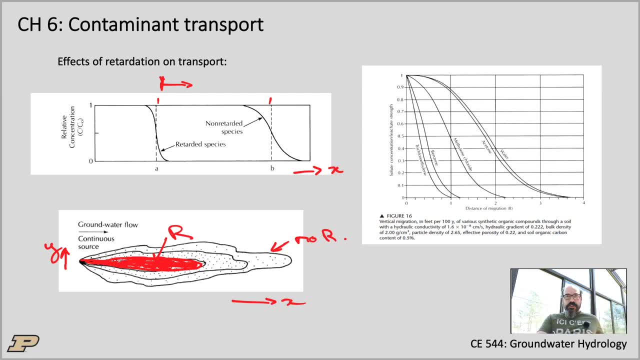 so in space you can imagine, the retarded species are just being, you know, less dispersed and less fast or slower. and the less dispersed is a little bit is not as intuitive as a the slower motion, right. so it's less dispersed again because some of it is absorbed, right? so if 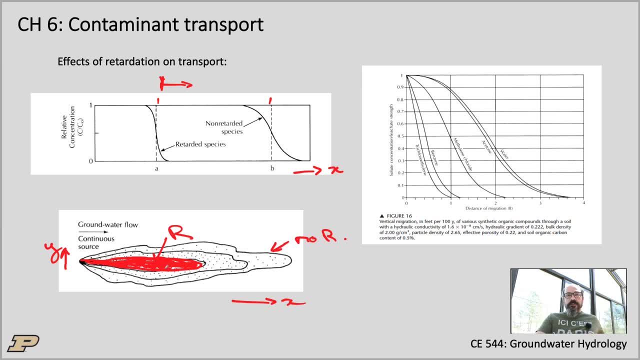 if you're a molecule and you're absorbed onto the matrix, now you can't disperse, obviously, right, you're stuck there. so that's really the effect on dispersion is really because of that, you know, being stuck, basically an amount of mass is like literally stuck and not dispersing at all. 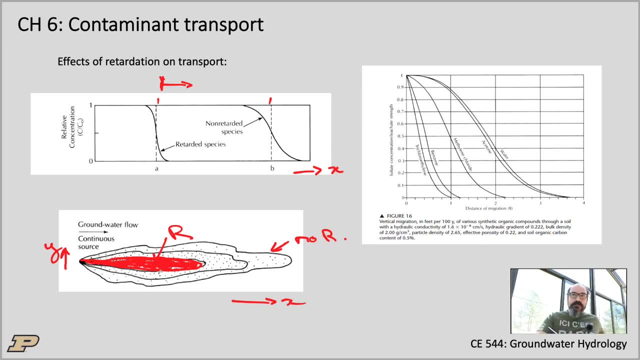 so the ensemble average, the mean dispersion, is less right. there's less material. actually, you know doing the random walk if you are moving away, because again some of it is stuck here on the right hand side you have examples of organic compounds being retorted and you can see the different compounds have different. you know retardation factors basically. so the 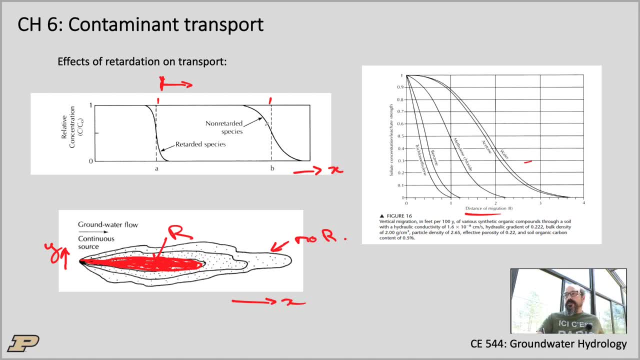 water again is up in front and again this is now in x, right. so this is in spatial coordinates like the space. so if the water is out in front, so this is the same as this left hand side front, if you will right. so if you have, you know this curve for water, you know different compounds. so acetone is retarded a. 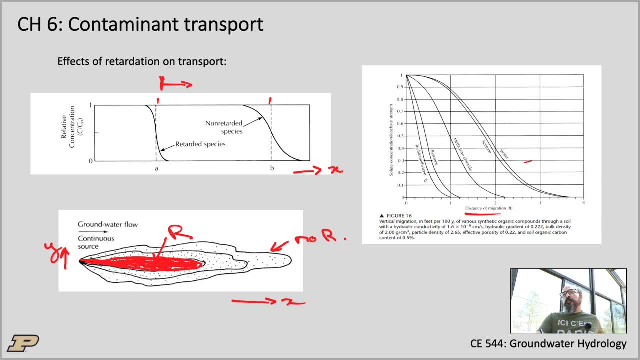 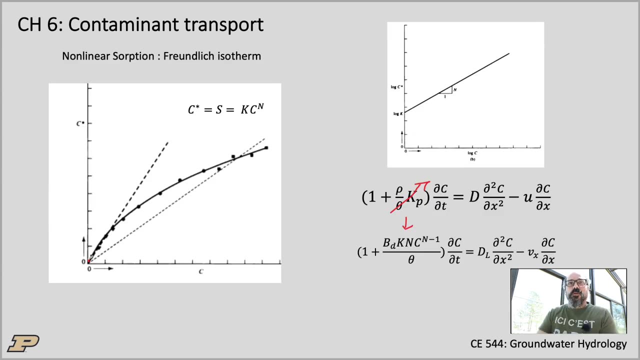 little bit, but not much, right, and you can see that different compounds have different retardation factors and trichloroethylene here is very much retarded, very tiny and very stuck there, okay, okay. so in real life we don't really usually have those linear isotherms that we've seen. 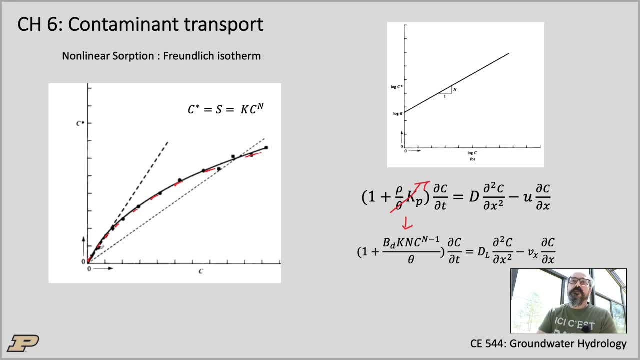 before. but what happens is we have non-linearity of the sorption. the reason is, you know, if you look at these linear isotherms like we had before, you can basically have infinite mass sorbing onto a finite amount of sorption sites, right? so if you think about it, like at high concentration, so at 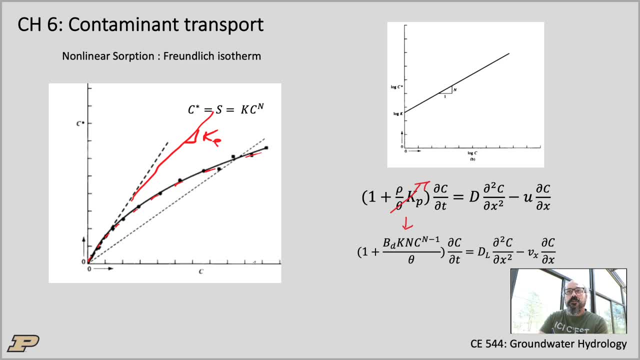 high bulk concentration in the plume, in the matrix, in the water. you should have, you know, some amount of sorbed material. now, if you increase the concentration a lot, right, at some point you saturate all your minerals. so once you're all your minerals are saturated right, it doesn't really matter how much more mass or how much more concentration you have. 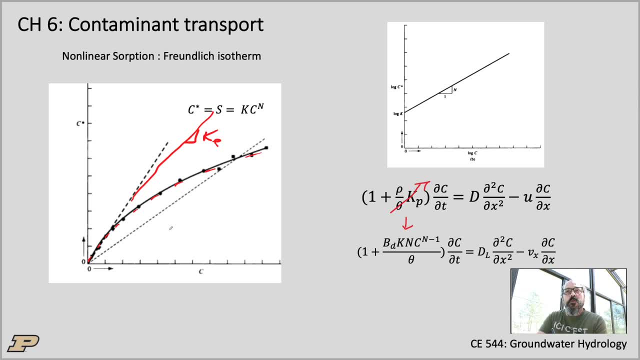 in the bulk, because everything is saturated, they can't just take any more, right. so there's a saturation process going on that is not accounted for by those linear isotherms, and that's why in reality, in real life, we always, almost always, observe those nonlinear processes right where again at 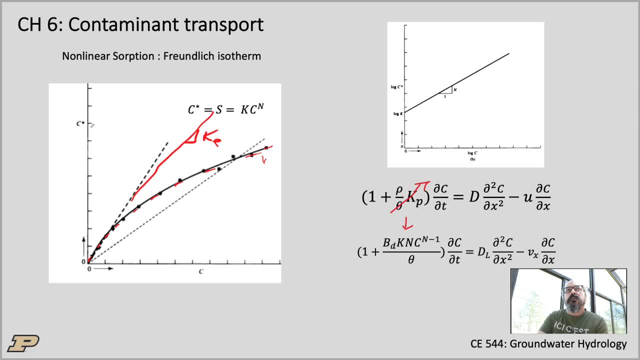 high concentration there is less, proportionally less right of the sorbed material. right again, because there's only so much we can stick in there. this is an example of, you know, a Paolo, basically isotherms. this is called a Freundlich isotherms. there's, you know, there's a couple that are common. there's different. 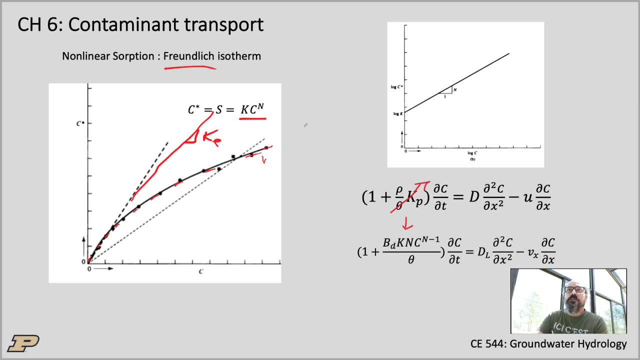 things that you could do, but this is just as an example, right? So let's say we have a Paolo relationship between the absorbed amount and the bulk concentration. Now you can see here on the right-hand side, obviously for Paolo, right? if you log the both axes right log-log-plot. 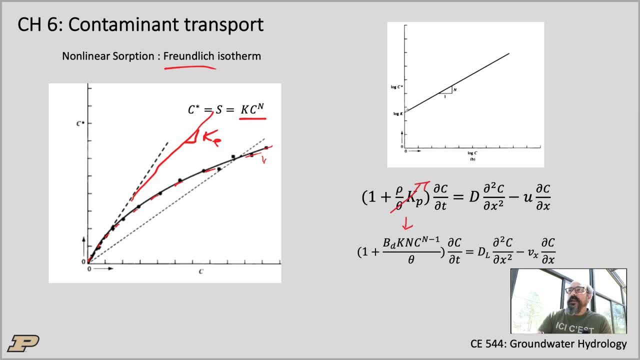 you get a straight line, and now the slope is n and the intercept is log k. So again, if you have that kind of data, you can just log-log, extract those two parameters and now we can finally calculate our retardation coefficient. But now, of course, right, because 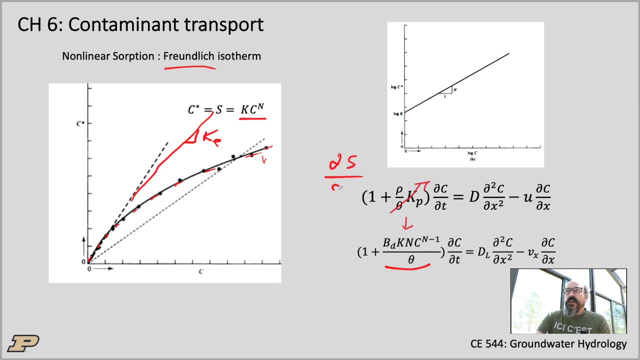 again ds, dc, right. so because the partition coefficient is by definition the differential of the absorbed versus the bulk, right, when we differentiate that Paolo thing right, we get this n, c and minus one here, and finally, you know. so here this is rho really. 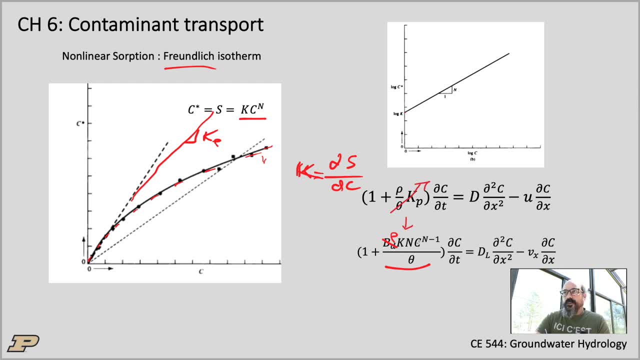 that should be rho. that's just the Fetter writing. But anyway, so you can see that it's a different partition coefficient. so this was the linear one, for you know. so you can compare. so now this is not true anymore, but we have this new thing, so if we have the data again, 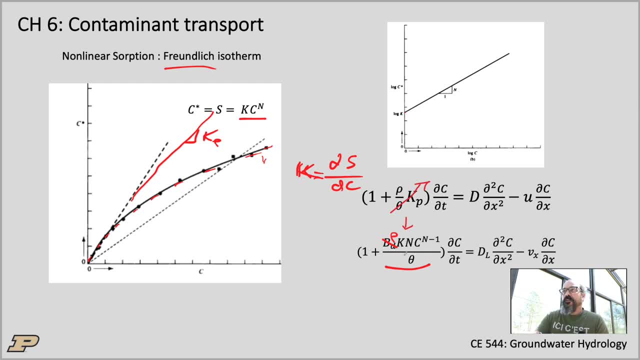 we can just, you know, measure n, measure k from the data, and then rho and theta are the same. so you can see that this is a slightly different retardation coefficient, but at the end of the day we still have some retardation coefficient. 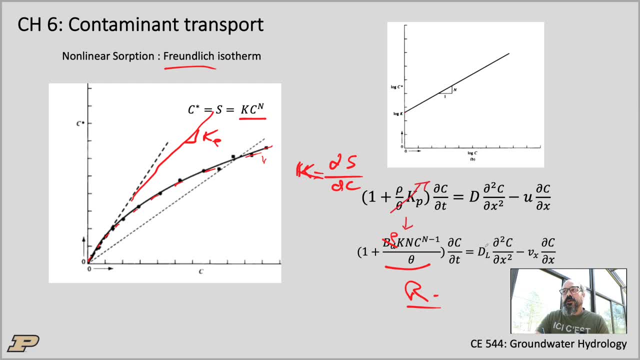 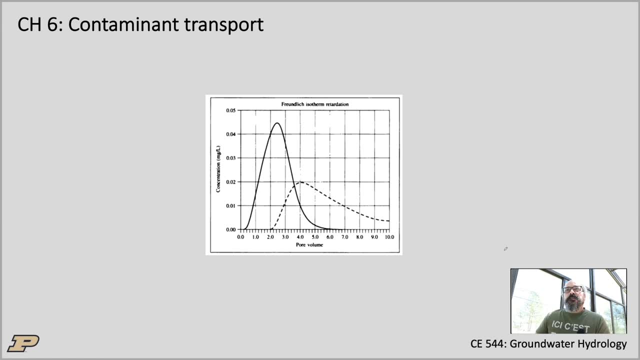 Right that we can just plug in and then the result is the same, that it is rescaling your dispersion and your velocity, essentially. Now, what is the effect of that? right, so we've seen before the effect of linear retardation is just to literally, you know, slow down. 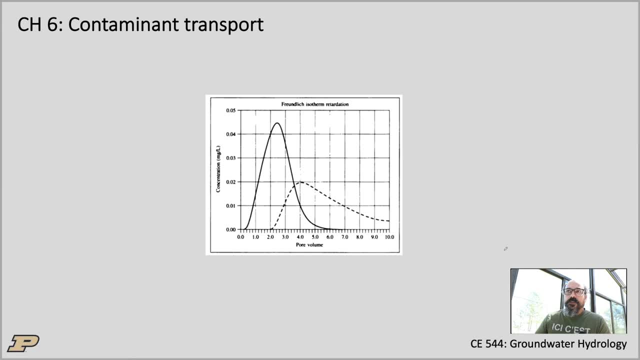 the transport. Here you can see that for nonlinear processes it's a little complicated because, again, the retardation basically depends on the concentration, right? so you can see here, Here we have the appearance of long tails and again this is that process that I talked. 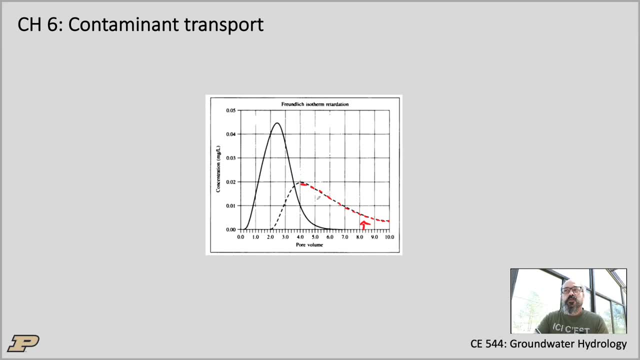 about before, when we have that clean water, flushing out the system, you know, towards the end. Well, now, because it was nonlinear, right, you have more mass. that is still hanging around, you know, after a long time. so not only there is a change in the timing of the 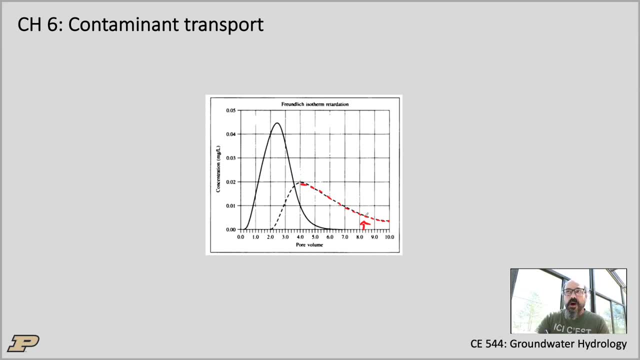 transport. but now we have a reshaping of the plume that is not, you know, obvious, right? so we are basically creating those long tails in transport, Those late-time elution that weren't visible for linear isotherms. so, really, here it gets. 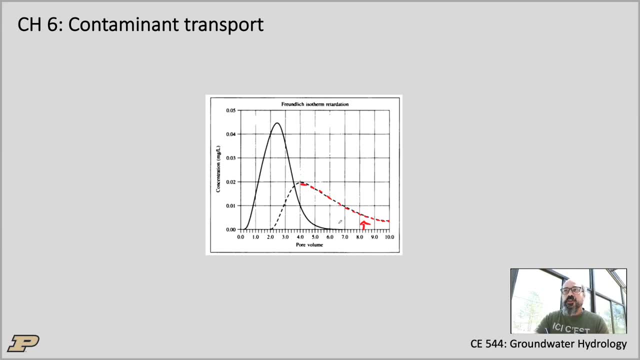 pretty complicated, pretty fast. Well, instead of just you know shifting, you know the transport in time. now you're actually reshaping the transport. so now you know. so let's say, for example, these were pathogens, right, cryptosporidium, for example, where you 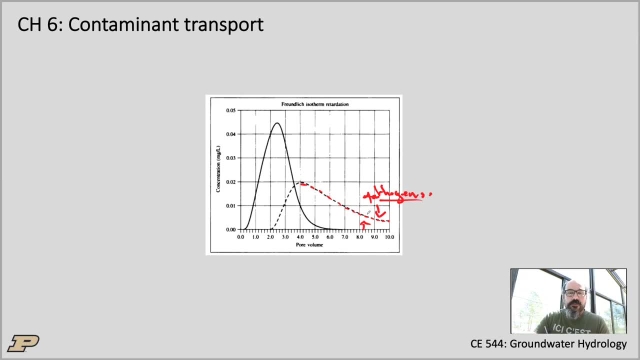 know, very, very low concentrations can be fatal, basically, or very dangerous for you know, very dangerous for public health. Well, now you know the risk is extended in time for a long, long time, right so now, instead of you know, after a few days you're done. 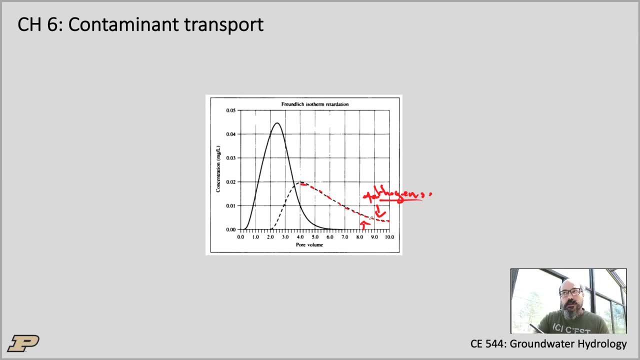 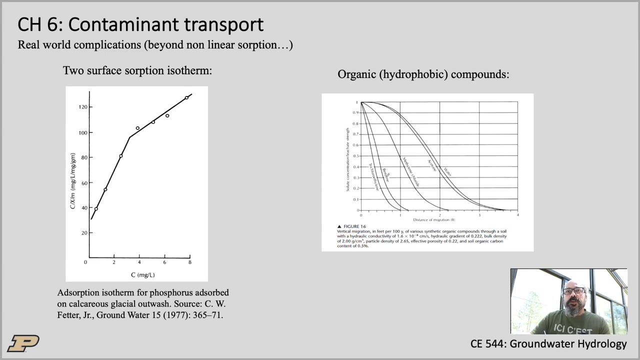 well, now maybe it's a few months because you have that lingering concentration that is coming out of that aquifer. you know literally forever, basically. So, again, nonlinear transport or nonlinear isotherm, nonlinear sorption, pretty tricky business, Okay. so other processes. 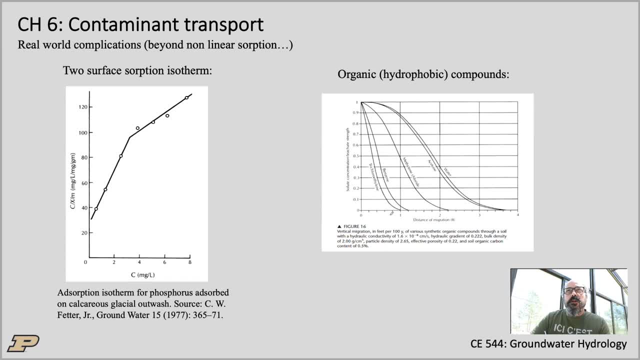 that can complicate the process. Okay, so let's talk about the sorption processes. Here on the left is essentially a dual or two-domain. you know linear isotherm, so it looks like a nonlinear, like just the one you like we've. 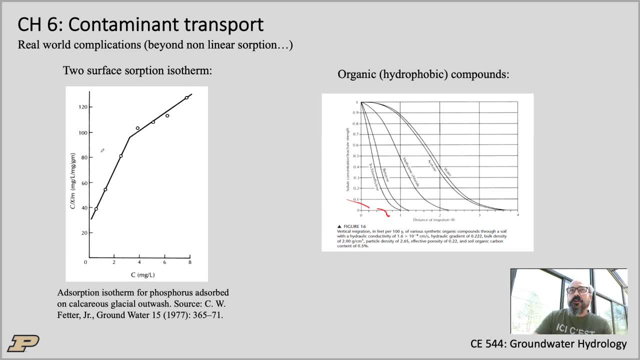 seen before, right? but here, if you look at this data, it's more like two different regimes with a regime shift in between, right? so this first one here, let's call it Kp1, and then the second one here, let's call it Kp2, okay. 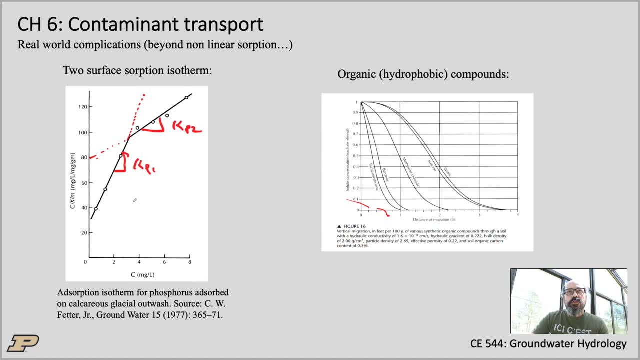 If we think of it right, instead of being due to just nonlinear sorption into one compound or one mineral in the soil, now we can have two different surfaces, basically having two different behaviors, right? two different linear sorption, isotherms, so each mineral. 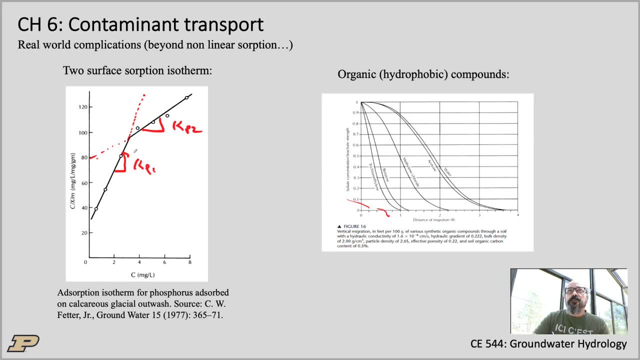 surface is different and then expresses, you know, different trends. so that's another example. So if you think of the natural formation, obviously they're complicated, right. it's not like simple one-step, One surface or one compound, one mineral. it's actually a bunch of different minerals. 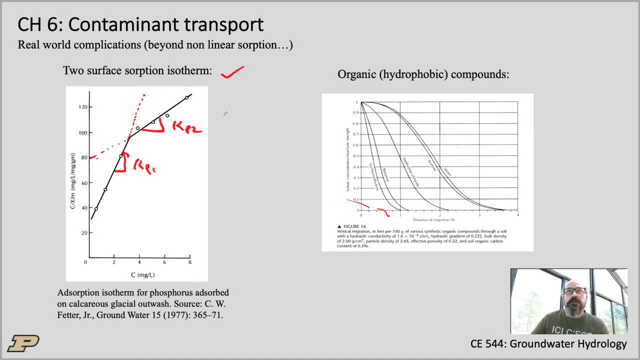 and organics, and you know the whole matrix is complicated, especially soils, for example. so you wouldn't expect things to behave, you know, linearly and kind of simply so. this is one example of a still somewhat simple two-surface sorption. you know problem. 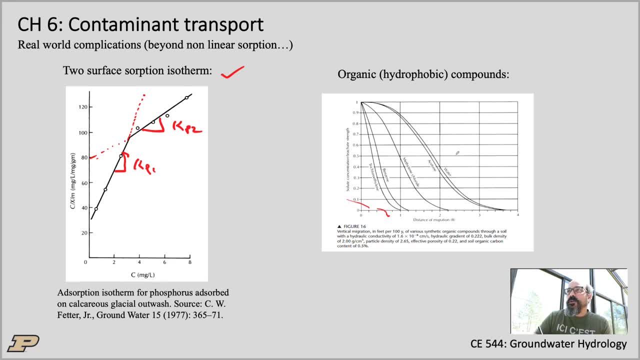 Here on the right-hand side. this is something I've shown before, right, with different organics being retarded more so the problem with organics- and I'll just say a few words, but you know I could do a whole chapter on this, obviously so organic compounds are, you know, essentially. 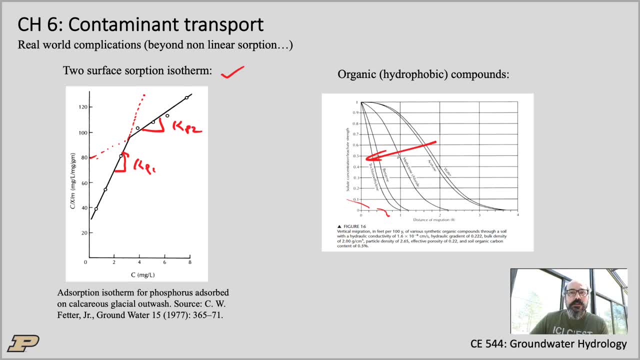 made of carbon, right, and carbon sticks to carbon right, so organics stick to organics. Think of, you know, oil and water, right, they don't mix. or oil and vinegar, right, they don't mix. so organic compounds tend to be attracted to other organics. so especially, 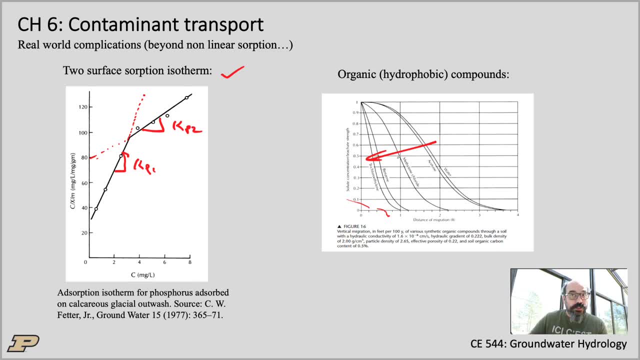 in soils, for example. if you have so the amount of retardation for an organic pollution- and these are very important Because you know all gasoline, gasoline products, right, all those are organic pollutions and when they travel through soils, you know their retardation- it will be conditioned. 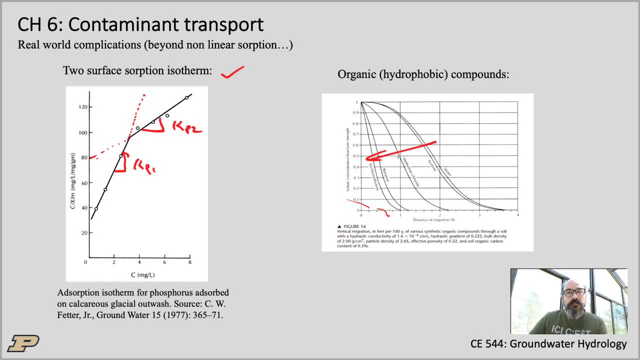 or will depend on the organic content of the soil itself, right, so the more organics you have in the soil, the more retardation of those hydrocarbon compounds you know you'll have. so this is really, really important and again there's a whole, you know, I mean. 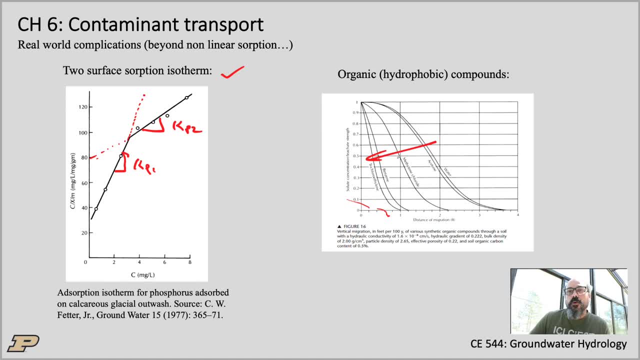 obviously this is really important. There's a lot more in engineering and remediation, so we could do a whole chapter on this. I'm not going to go too much into it, but just remember that basically the retardation factor for organics depends on the organic content of the formation. 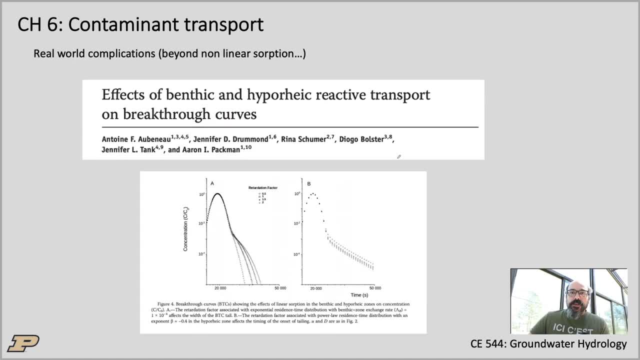 Okay, and finally, just sort of to bring this back to you, know what I do for a living? I guess what I do for research. this is an old paper of mine showing the effects of hyperreactive transport on breakthrough curves. so again, hyperic is what you know is basically groundwater. 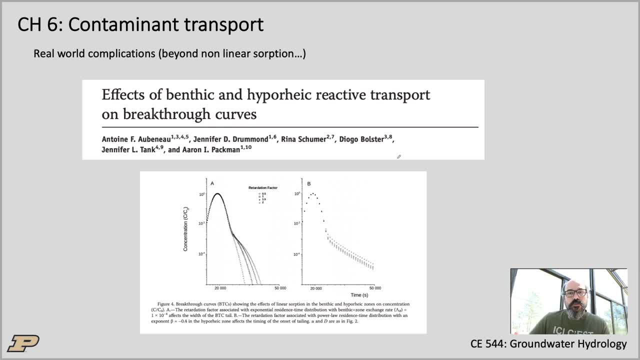 surface water exchange. so the hyperic zone is that zone around streams and rivers in the sediment right. so there's, you know, obviously rivers flow, you know, in alluvium a lot of the time and there's an exchange of surface and groundwater. you know, at the 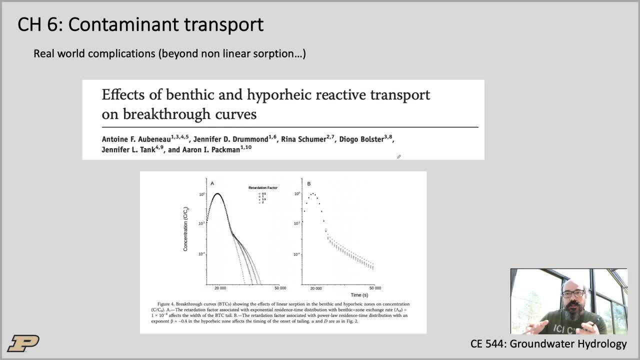 interface there, right, so groundwater comes into the river, but then the river also, kind of you know, contributes water to that hyperic zone, to that zone just around in the sediment right, The sediment just around the streams and rivers. 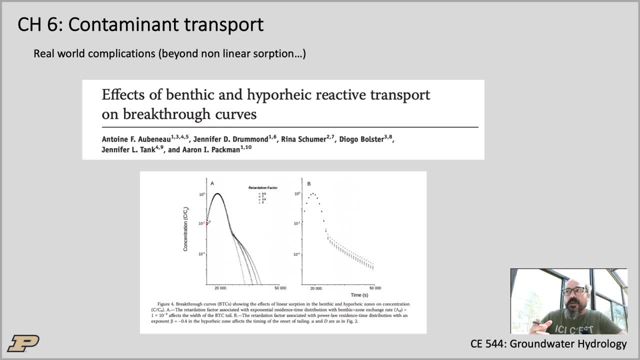 Now here is a couple examples so you can sort of recognize those pulse right, the sigma or the dispersion, I should say the velocity. it's called dispersion, so you can sort of recognize that Gaussian bell-shaped curve on the log-log plot. but then here at 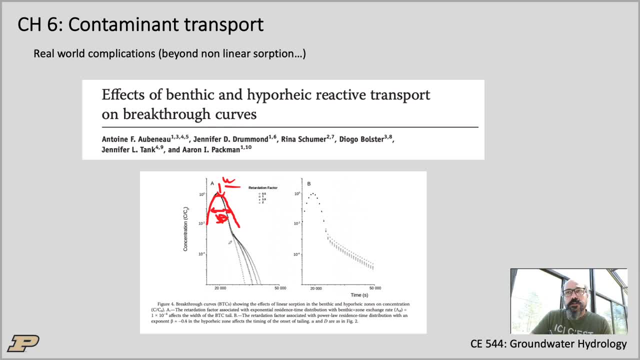 the bottom is really the impact of that hyperic zone, basically of that water that went into the sediment right and then back out. so in the sediment, you know, it goes a lot. it goes a lot slower, obviously, than the river flowing by. so in the sediment it goes. 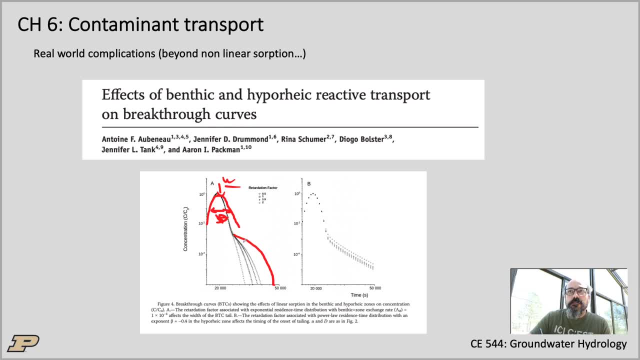 slower and this is why we have those tailing behavior, basically at late time, because this is some water that went into sediment. Now, inside the sediment, what can happen is, you know, retardation can happen, right, and so this plot here just shows, you know, different compound for different retardation factors. 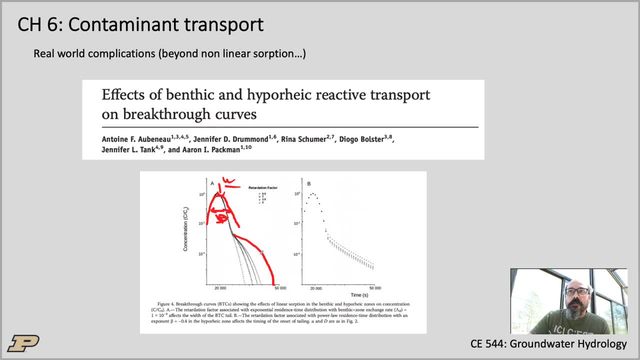 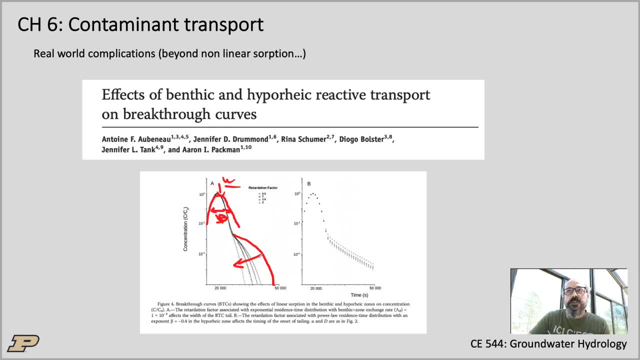 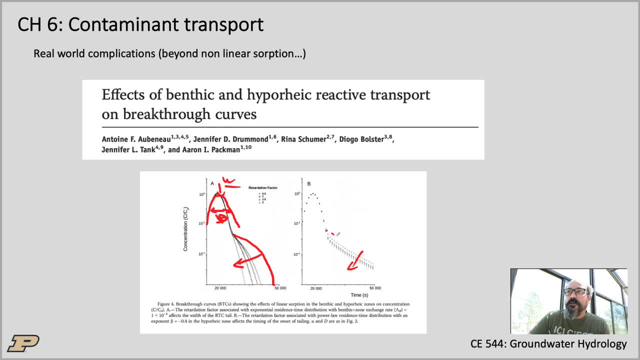 So if the water is, you know, up top here, this was water. Now the retarded compound comes out of this sediment below the stream. you know, later and later and later- and that's really the point I'm trying to make here- is that those 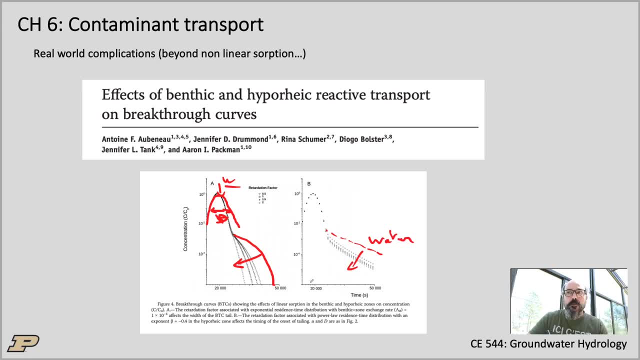 you know there's a lot of real world applications that you wouldn't think about for retardation that are really important, right? so a lot of superfund sites have you know compounds that are stuck there because of retardation, that are stuck on the matrix. if 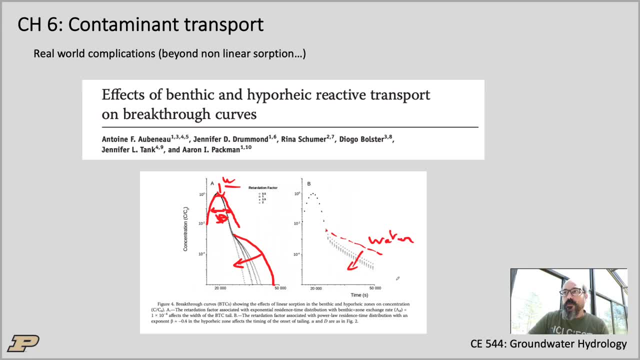 you will like that absorb, you know, onto those minerals or organics in that formation. and the question to the environmental engineers essentially is how can we get them out right and what can we do to help? or sometimes, you know, it's the opposite, where you have a plume of a pollutant that is 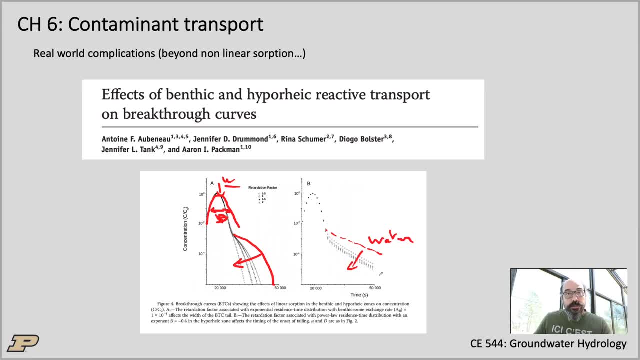 moving through a formation or through an aquifer and you'd like to slow it down. right, so sorption can also be used in remediation, to sort of: you know, what can we do to slow it down? basically, can we add something to this formation to precipitate, to absorb to, you know, eliminate? 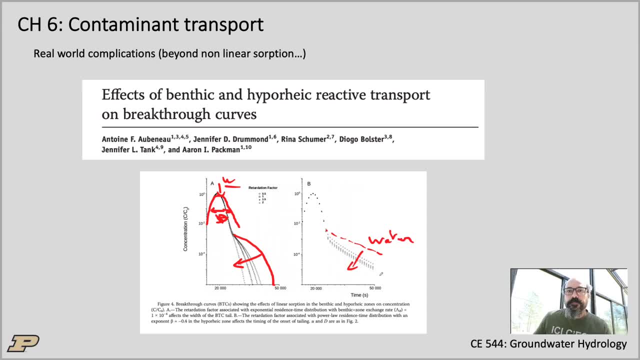 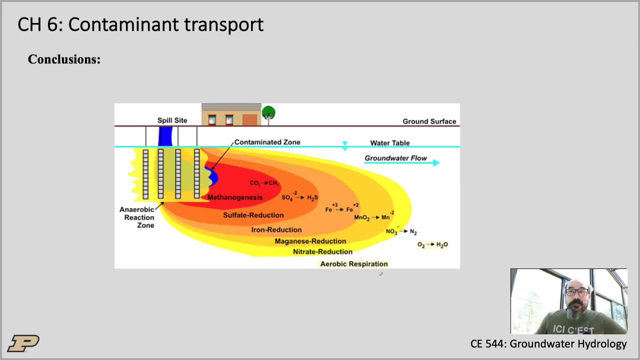 this pollution, or slow it down at least, so we can get you know mechanical solutions downstream at some point. okay, finally, i'll conclude on this. so next time i'll do other types of reactions, so degradation, reduction reactions, and this is an example where you have a plume right and you can see that, depending on 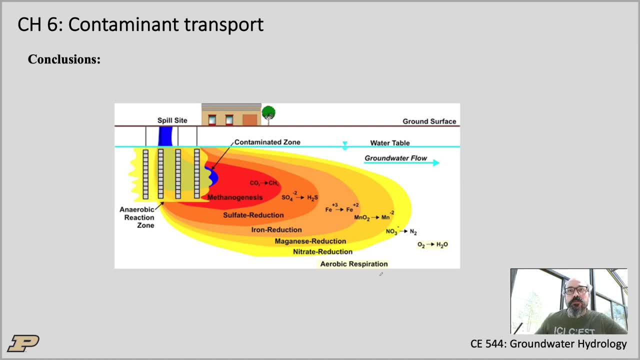 where you're at, uh, physically like, especially in the plume. you have different sorts of reaction and this is your sort of standard, right, red redox, uh, france. so you have, you know oxygen is used uh, all the way out. right, there's oxygen here. so this is the first thing that 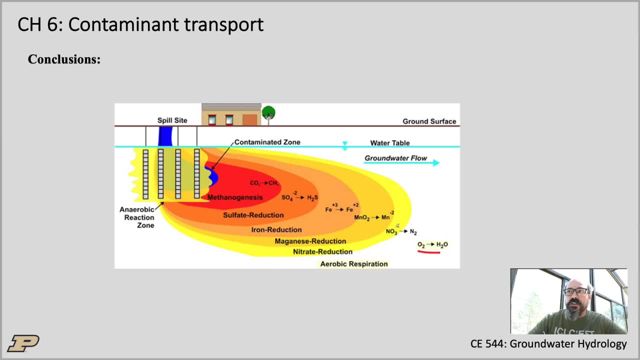 that goes basically that we respire, but then when this oxygen is gone, right, we get the oxygen basically from other compounds, and this is like denitrification is the next one here. so we get the oxygen basically from the nitrate and once we remove the oxygen from 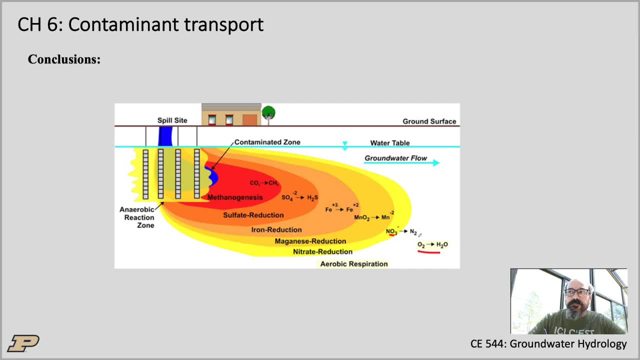 the nitrate that gives nitrogen gas. right. here you have manganese oxides, right. so once the nitrate is gone, right, there's no more nitrate. well, we go down the ladder, right. so now we use manganese to get our oxygen. now the oxidative power. so now there's no more oxygen. basically, no more oxides. 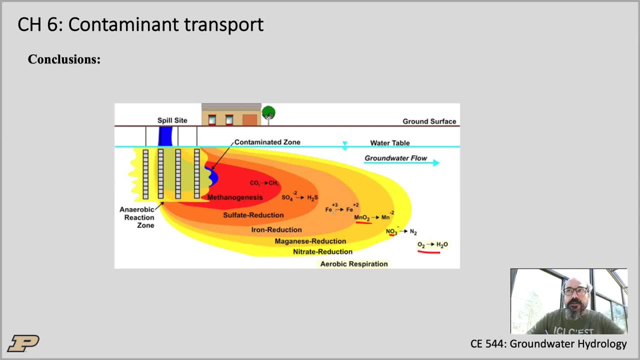 so now we have to start reducing. you know other stuff. so this is iron, and iron is a typical one. i really like the iron example because when you see a spring, a groundwater spring, so when you, you know, walk in a wet forest somewhere right and there's a seepage of groundwater. 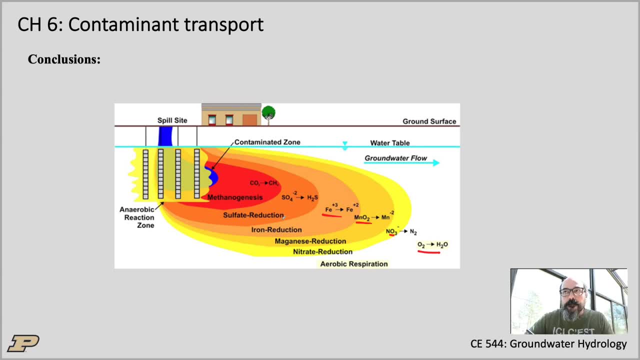 basically that you can sort of tell by how swampy that place is. you can. you can actually see the iron precipitate as iron three. when it comes out of the ground it's usually reduced, so that would be iron two. there, right, it's reduced. it has that gray or green gray sort of color, and when it comes, 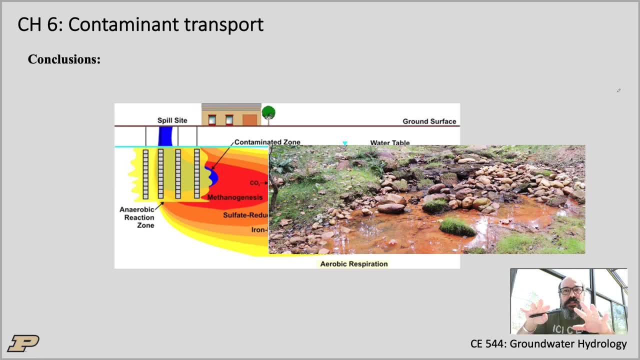 up to the atmosphere, right it's. it gets in contact with the air, so the oxygen in the atmosphere, and all of a sudden it gets oxidized into that rust, right into that red color and you can literally see the red iron precipitates around those little springs and stuff. so this is a 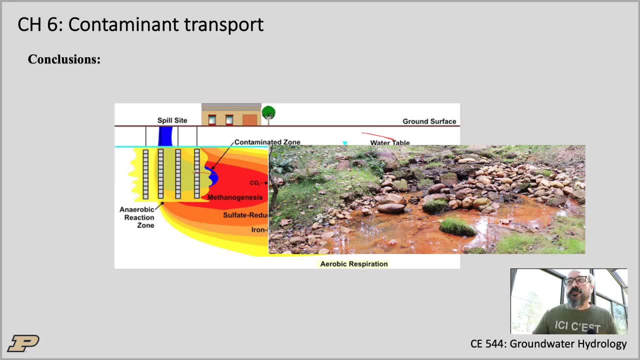 pretty interesting phenomena. so this is something we'll describe some more in the next lecture, where we'll get into degradation and decay. all right, thank you very much.